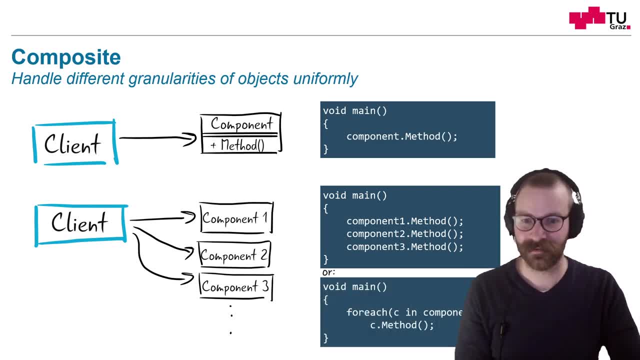 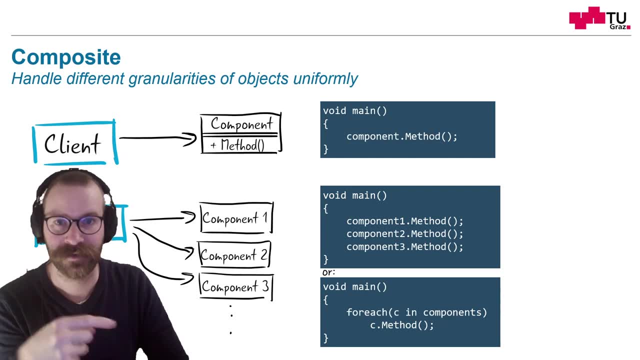 for example. Then it can look like this: Let me move to the other side. Here we are just looping over all components and calling the method we want to call, But the problem is now: what if we don't know how many objects we will call? How can? 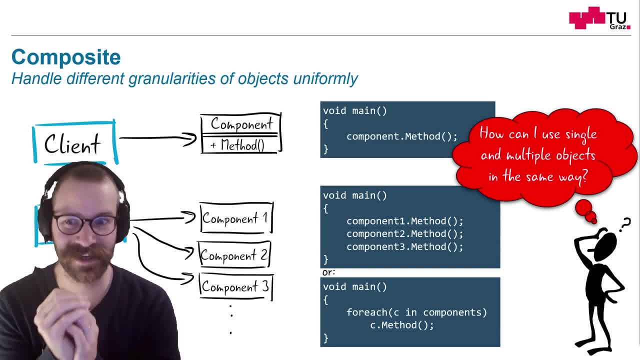 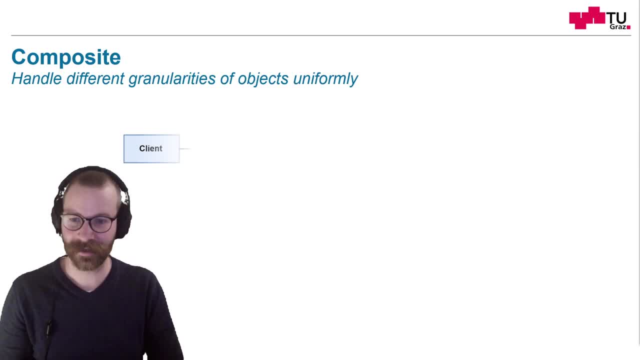 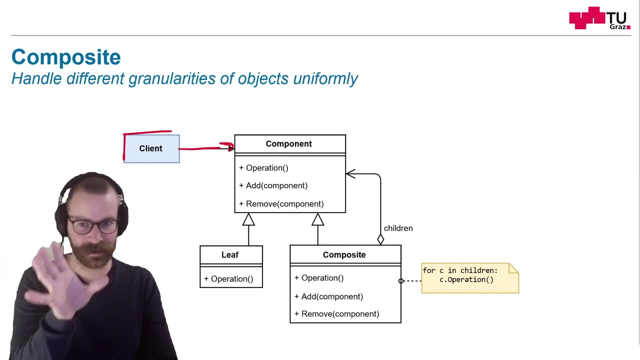 we use single and multiple objects the same way. That's the problem we want to tackle with composite. How does this look like? Like this: We have a client which is calling some method Here Which is calling some method, some operation. 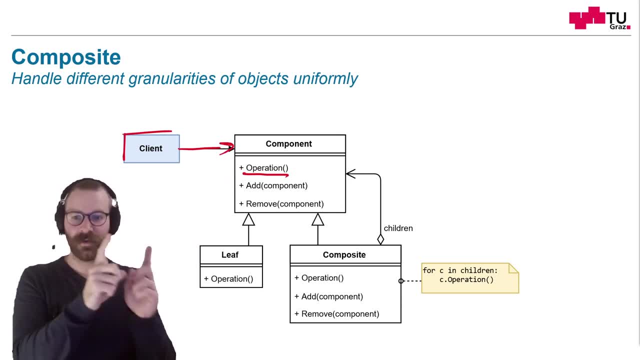 All is from the component. We have now two variants, Two possibilities. Either we are on a leaf. we are calling the actual object which should be called. This is the first option. Or we are on an aggregate, We are on an intermediate leaf. We just have the purpose of rerouting this call to another object. 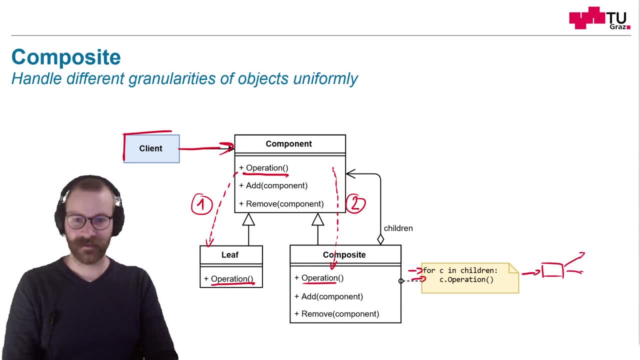 to an actual label And as you can see now, it works perfectly. It is not just to call every object, It's just the combination of called objects. It even works for希ilton. This is the mean that to an actual leaf. then this will be rerouted over and over again. the 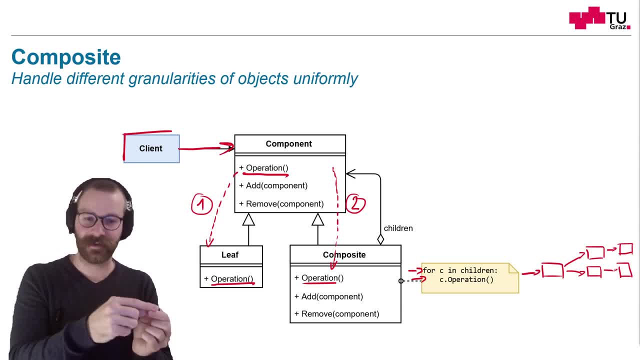 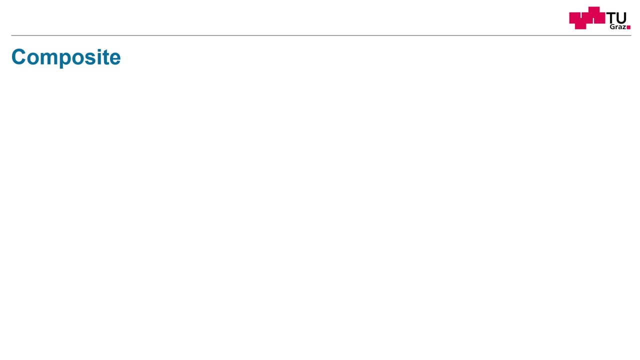 composite part has the purpose of transferring the coal to all its children. in order to have children, we have to add these two methods. first, we want to have a list of all children and we should give the possibility to add or remove further components. what can we do with the structure? first of all, we, as a 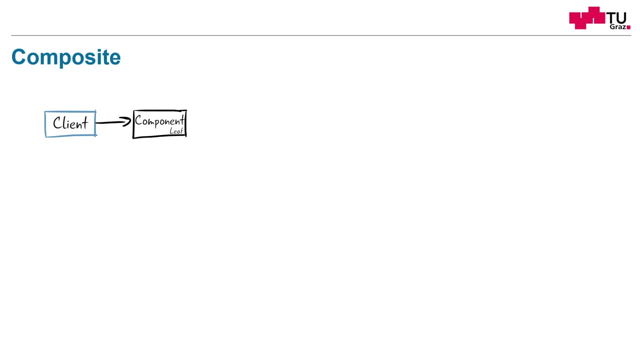 client can just call the methods from another component if this component is a leaf. we are done ok. in this way, single objects are considered. if a client calls the same methods from a component which actually is a composite, what happens behind is this call gets transferred over to another composite and maybe to another leaf. 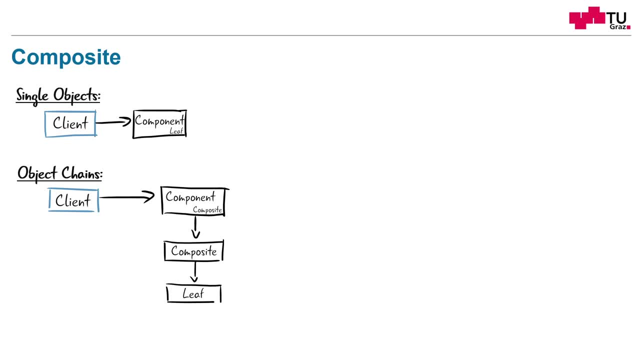 We can consider object chains now, And for the client it makes no difference if we call a single object or an object chain. And even further we can call whole trees of composites and leaves. This can be arbitrarily structured. In this case single chain is just a very simple tree. 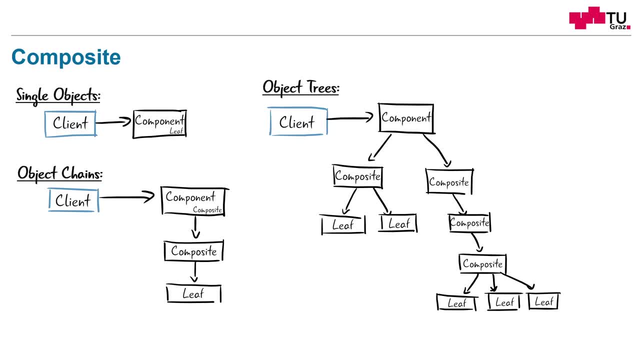 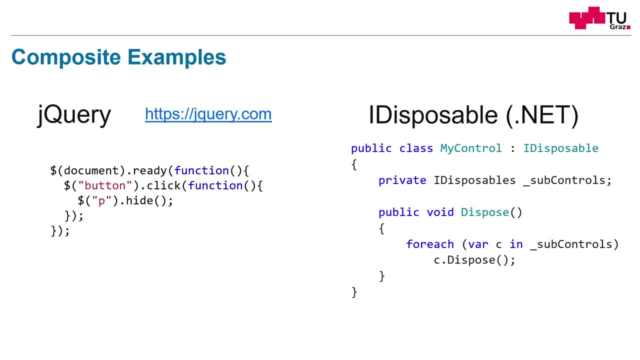 But this tree can be arbitrarily complex, But for the client it doesn't make any difference, because the client just calls the method, as he would do in single objects. This is what we wanted. Let me give you two examples: The one is from jQuery and the other one is from the IDisposable interface in NET. 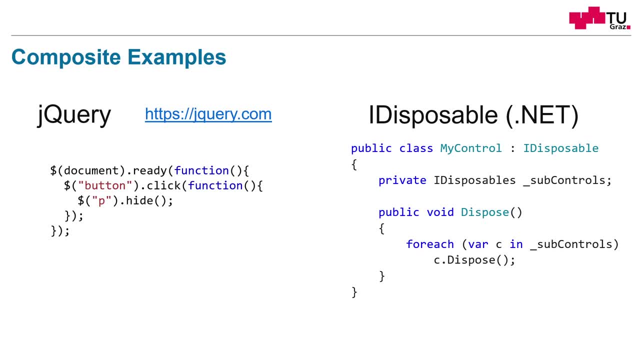 Let's look at the jQuery example first. Here on our main document we add another function to the ready event, And in this function- in jQuery this is called the selector- We select all button elements in our document And this can be one button. 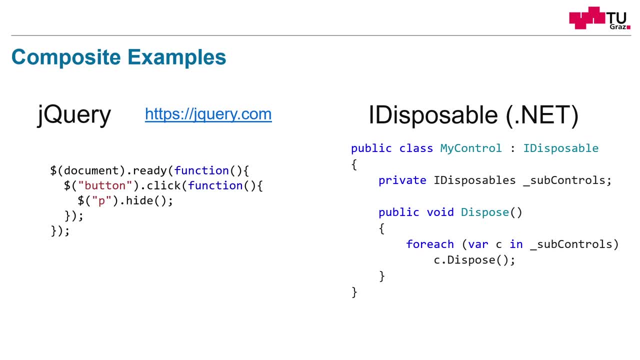 For example, a save button on a website, Or these can be multiple buttons, But regardless of how many objects there are returned, We add to the click Click event another function which calls the hide function, on all paragraph elements, And again it doesn't matter if there are multiples or if there is only one p-element on our website. 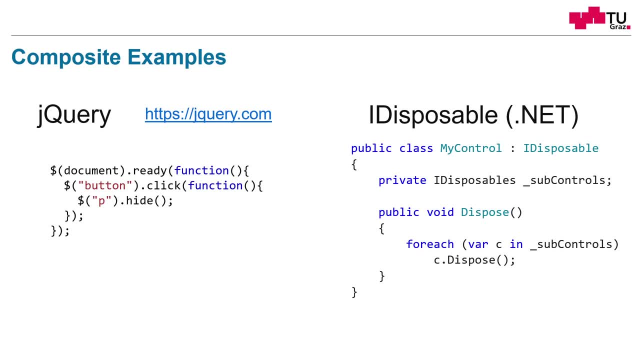 The IDisposable interface in NET also incorporates the composite idea. If you call dispose on an IDisposable object, then this method actually does two things. First, it cleans up any elements. It cleans up its own resources. In this case, we have no resources in this control. 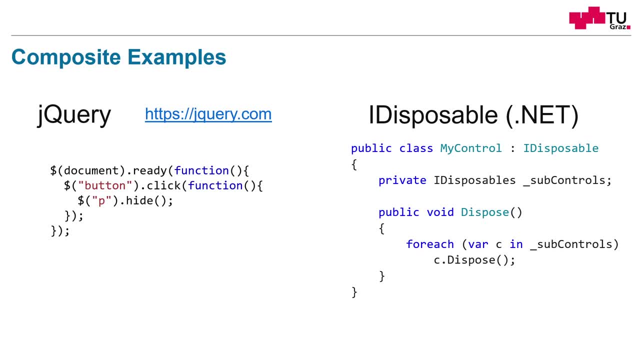 But it also routes this dispose command or this dispose method call to the sub-controls. We can see that a single call to dispose actually executes multiple calls on all sub-controls And these also reroute this call to the sub-controls. Let's talk about individual attributes now. 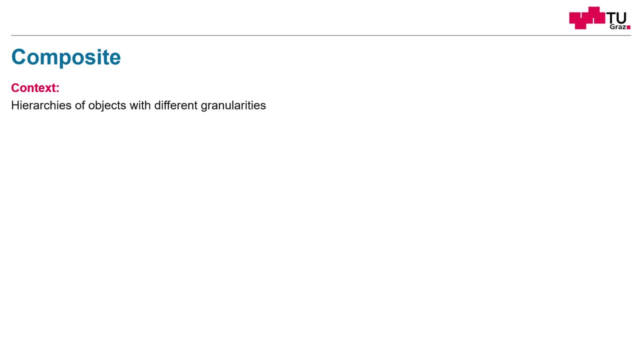 What is the context? We have object hierarchies with different granularities And the problem here is we want to treat them uniformly. We don't want to make a difference between single objects and multiple objects And maybe also different hierarchies of objects. 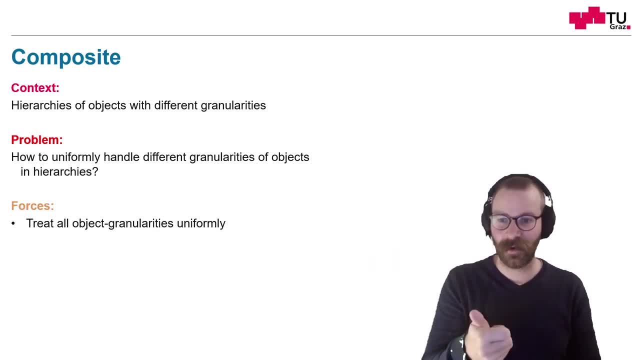 What are the forces here? First of all, we want to treat all object granularities uniformly, Then we want to reproduce them And then we want to replace them. We want to represent arbitrary object hierarchies, If it's a list or a tree or any kind of object hierarchy. 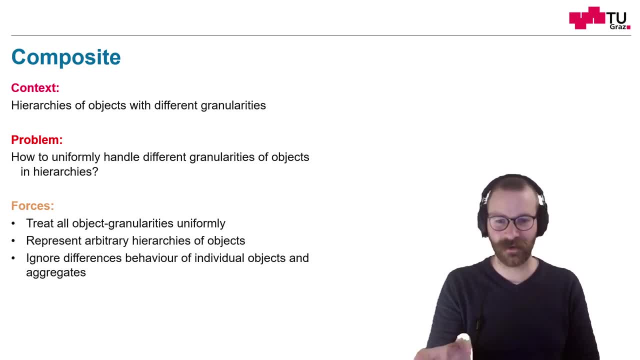 Then we want to ignore the differences between individual objects and aggregates. We don't want to create special methods for individual objects and multiple objects, And of course, so that this all works, we also want that method calls are rerouted to all objects. 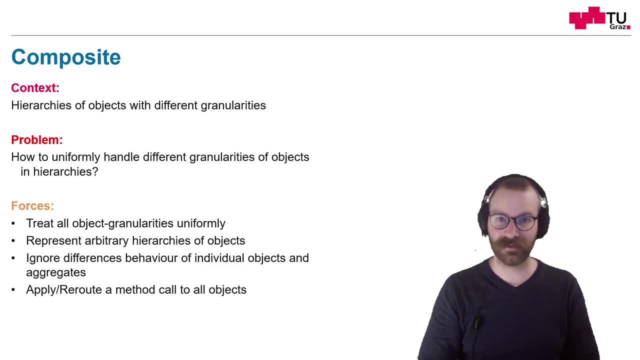 Which are interesting to all objects which belong to this hierarchy. The solution to this is to firstly define a common interface for all granularities, to manage children and call methods. This is the composite interface. This is the interface which supplies the original methods we want to call. 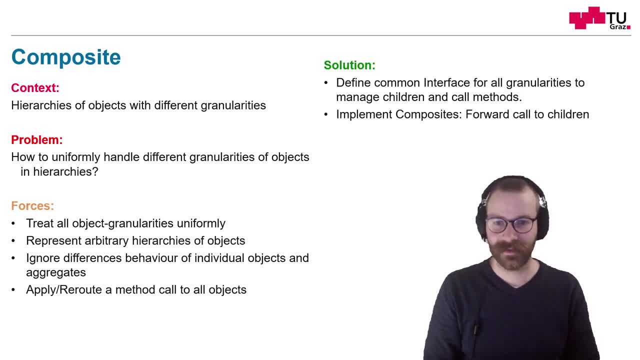 And which supplies this add and remove children. Then we have to implement the composite Which just forwards the call To the children, And then we have to implement the actual children underneath Here. there is no rerouting to further children. Then the call is directly executed. 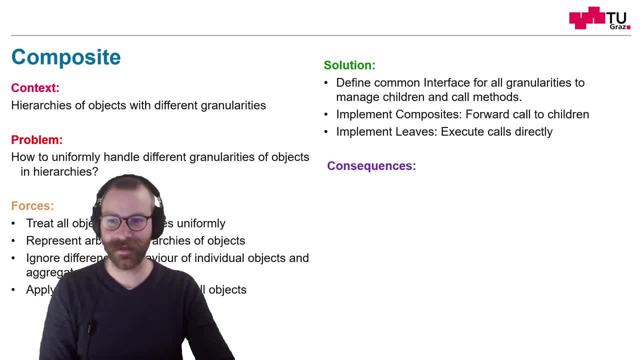 What are the consequences now? Let me just move out of the way. Firstly, the composite defines hierarchies of primitive and composite objects, So we can create arbitrary hierarchies. Furthermore, it's simple to use for the client. It doesn't have to make a difference between single objects and multiple objects. 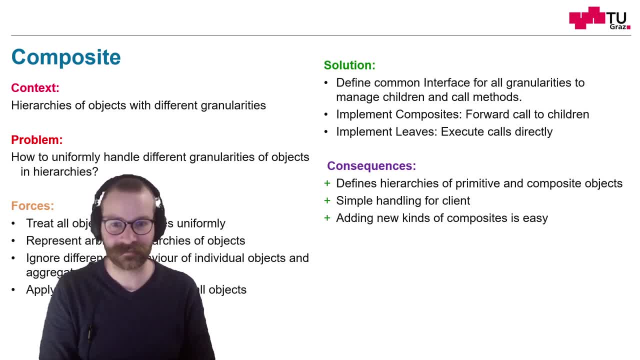 New kinds of composites is easy to add, But there is a liability. Where should the default implementation lie? In the parent class of the composite, For example, adding and removing children- Or should it be in the composite? If you implement it in the parent class, then also leaves have the capability to add and 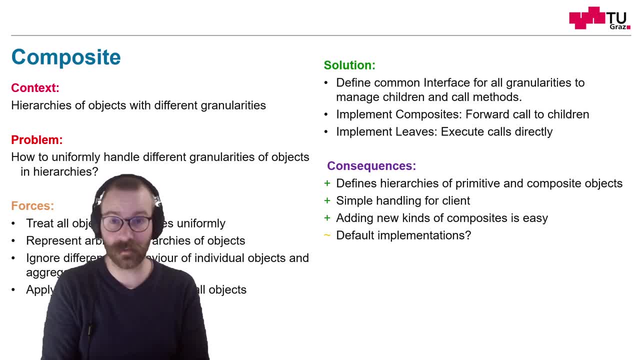 remove children. Maybe we want to do this, Maybe we don't want this behavior. Furthermore, should we create only references to children, Or should we also implement a back reference to the parent, So that we always know in which hierarchy we belong to? 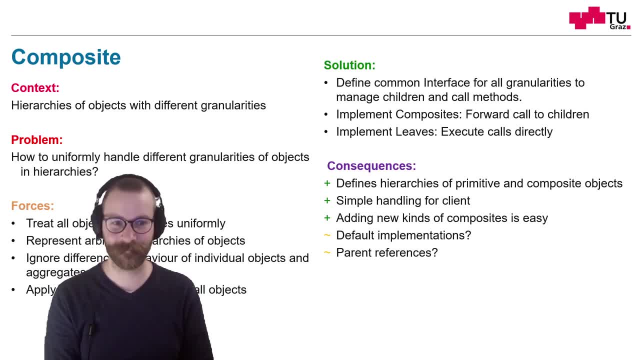 And that we can change and access the parent hierarchy. What about changing roles? When is a leaf a leaf And when is a composite a composite? For example, Can we just add some changes From children to a leaf and then it automatically gets a composite? 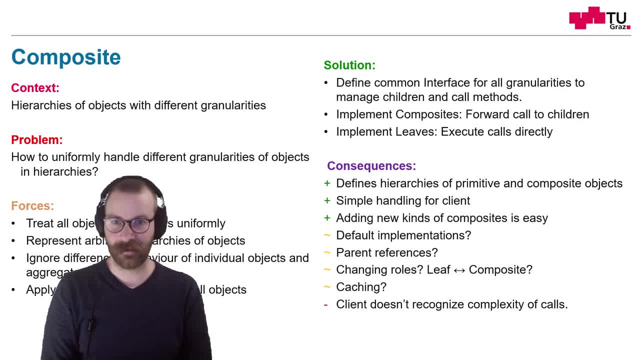 What about caching? For example, if you want to do some calculation over a complex hierarchy of objects And you say that's way too slow, Maybe I just store the results from my children And if I already have a calculated result, I just return this result. 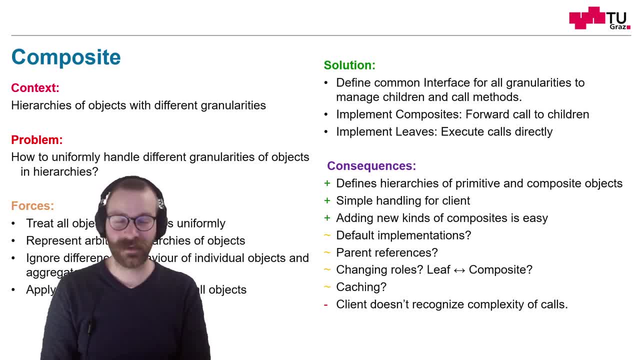 Otherwise I calculate it, But we don't know when some things in children may change. Therefore our cached results could be wrong. The observer pattern could solve this problem. We get informed when children change, And every time a child changes we completely delete our caches. 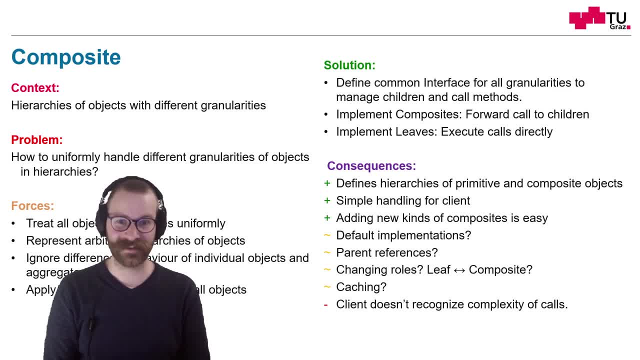 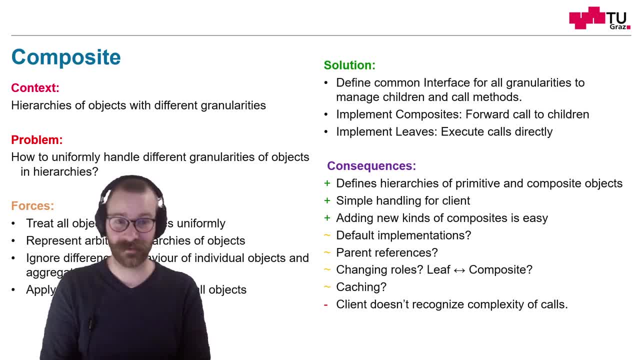 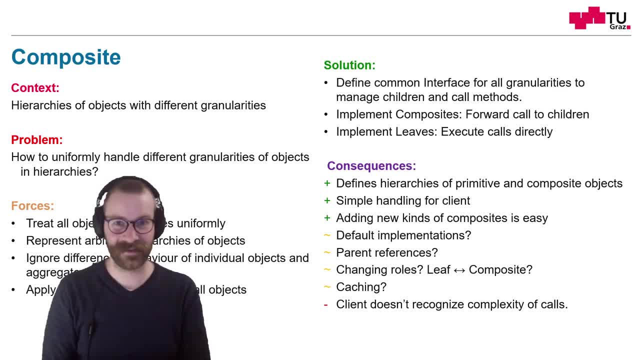 the hierarchy behind. Maybe it's a linked list, A simple object chain, Or it's a whole tree. You could have potentially high call hierarchies. Instead of just calling a direct method, you have a call which calls another call which. 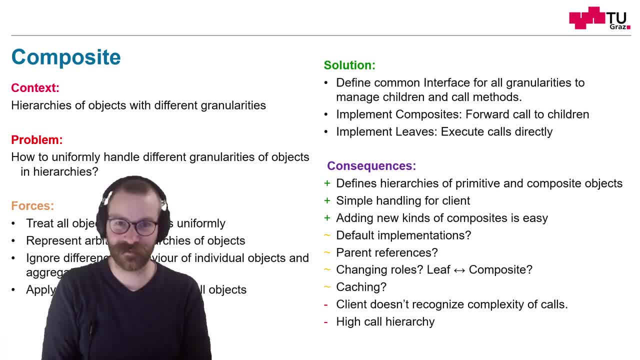 calls, another call… Every time you have a new layer of function calls. But its a Skype call. Maybe your pray will go to a great cloud using it, But for now we are on cloud 9.. It's desktop. If you have made it to cloud 9 here, it should and should not. 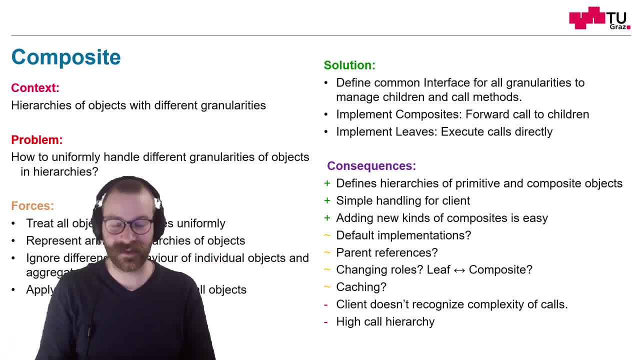 If you have been to cloud 9, this will work. It just happens that every time you create a Himself following example in the right tab you'll see the middle В? рlcf cakes are really stack gets bigger and bigger and bigger and maybe the stack could run out of space.